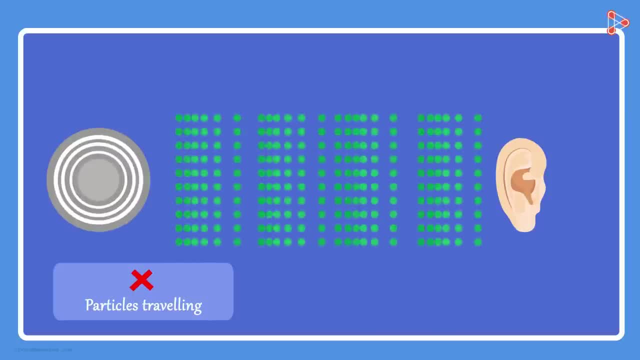 We see that particles of the medium are not travelling from the source to the human ear. It is the disturbance produced by a source which is travelling in the medium. The particles are merely oscillating from their mean positions. This disturbance, created by the vibrating object in the medium, is what we call a sound. 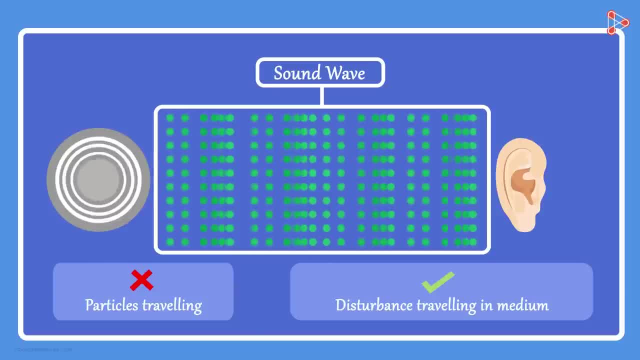 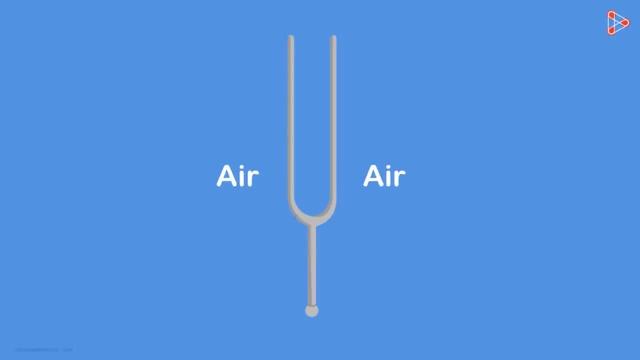 wave. But what does this disturbance look like? Let us study this with the help of a tuning fork. Here we take air as a medium of propagation. Here we have a tuning fork made up of steel. This shows the initial condition of the air particles of the medium when the tuning fork 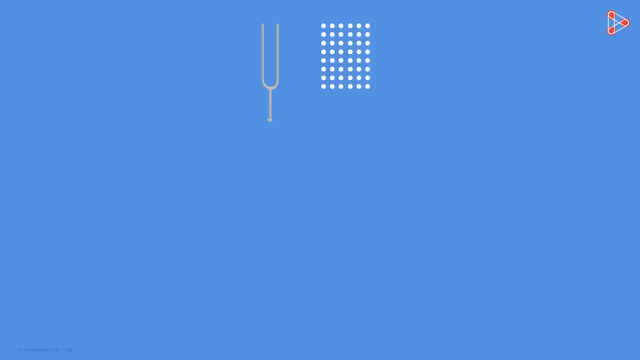 is in its original position, ie when tuning fork is not vibrating. When we strike its prong on a rubber band, we start hearing a sound. How does the sound travel through the medium? The two prongs of tuning fork are vibrating. 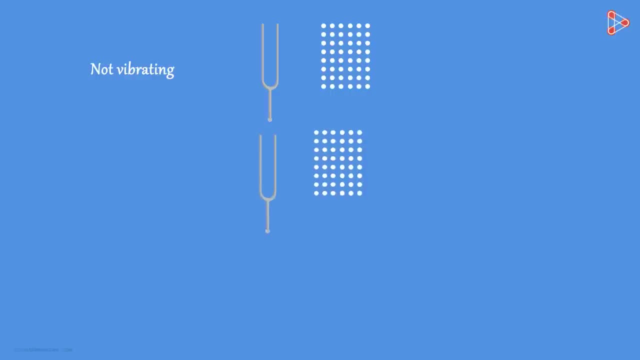 Let us concentrate on motion. of one of the prongs, first Say the one on the right. When it is away from its mean position, it pushes and compresses the air particles around it. This creates a high pressure region, also called compression. This compression travels in the medium as a disturbance. 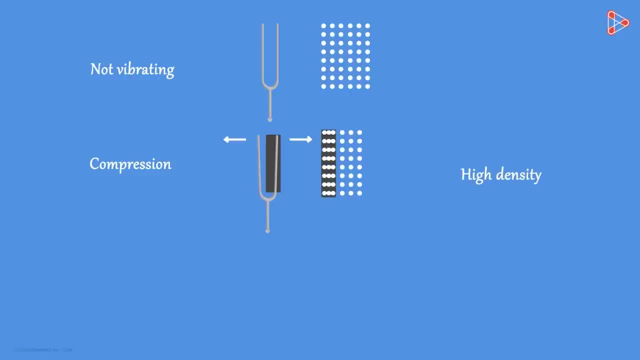 Here the density is high, ie The particles are very close to each other. The air particles are very close to each other. When the prong comes towards its mean position, the pressure on the right decreases and keeps on decreasing further as the prong continues its motion towards left. 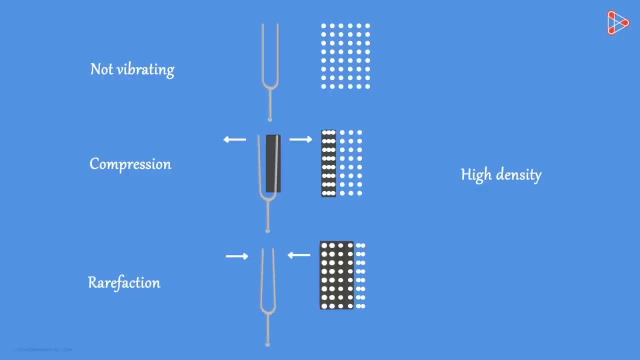 This creates a low pressure region, also called as rarefaction. We see that at this point the compression in the form of disturbance has reached this region. This rarefaction also travels in the medium as a disturbance. Here the density of particles is less, ie. 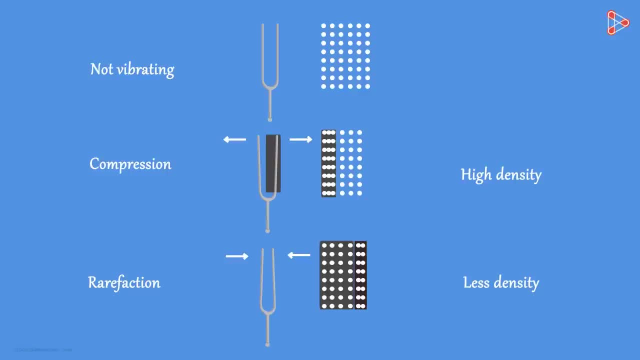 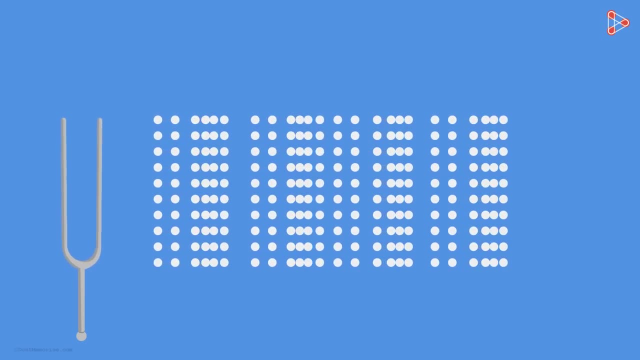 The particles are far away from each other. As it continues to vibrate, we get a series of these compressions and rarefactions. This continuous sequence of compressions and rarefactions is what we call sound waves. Yes, the sound waves travel in the form of compressions and rarefactions.